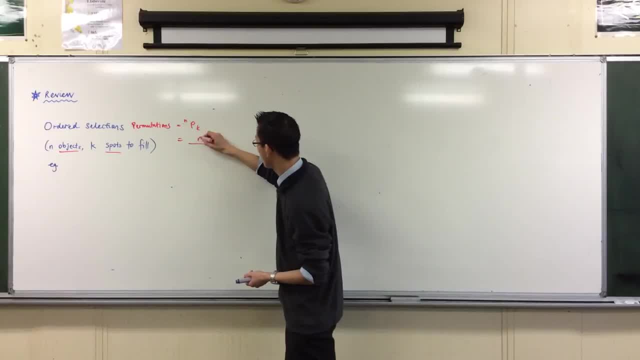 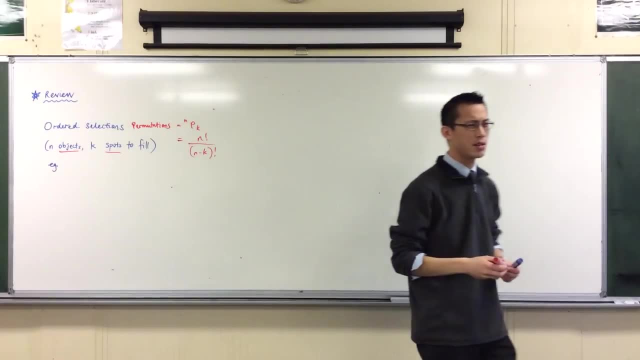 What's the fraction? What's on the top? N factorial good. And then we're dividing by N minus k- factorial right. Why is it N minus k? So the idea was you had your spots, By the way. I keep doing this. 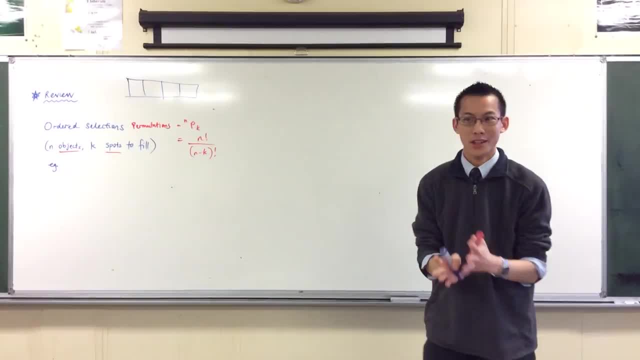 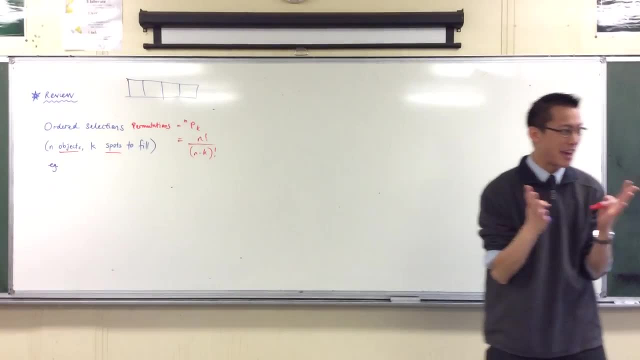 I hope you're not getting sick of it. It's such a useful tool. Nine times out of ten, when someone has come to me as you're working along, you're like: I have a question. Nine times out of ten. my explanation begins. 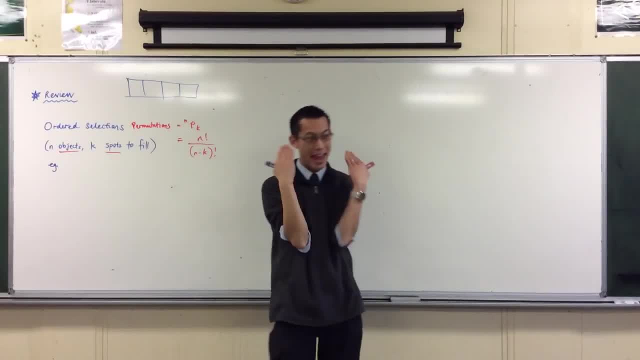 well, think about, and then I draw this either on the board or in my head, because it's just such a useful way to work out what's going on and why. is my answer wrong? So you start off with N different choices. 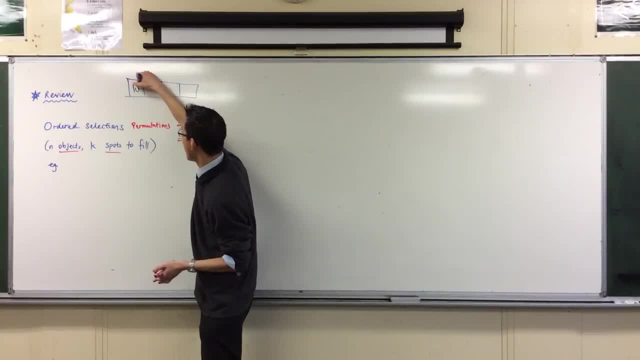 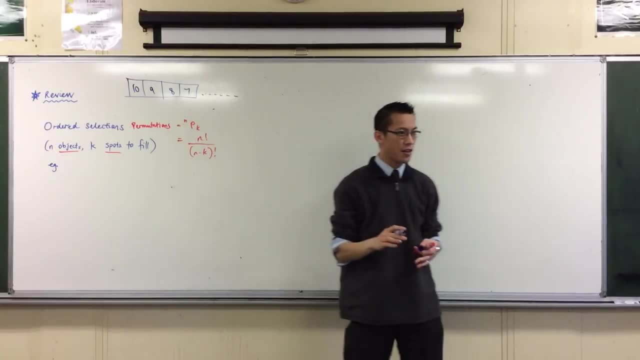 because that's how many objects you've got to choose from, Say 10.. And then you go well, 9, and then 8, and then 7. And the thing you have to divide by the number of factorials, that's missing. 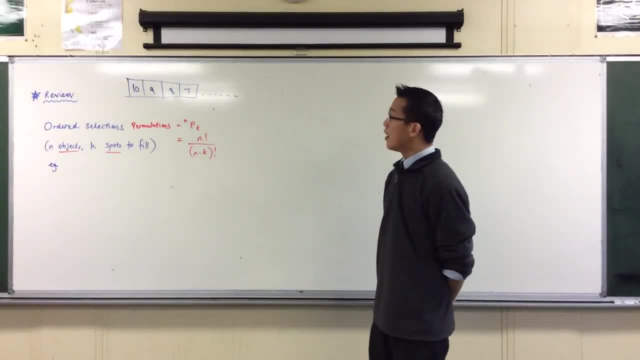 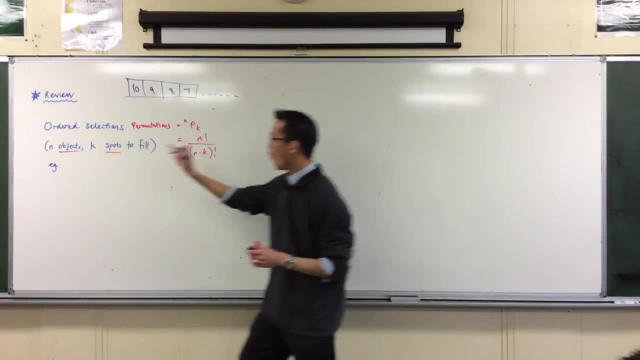 is N minus k factorial. In this case, I guess it would be 10 minus 4, which is 6 factorials. So we're okay with that. Now the examples we looked at, where order matters. What were the examples we looked at? 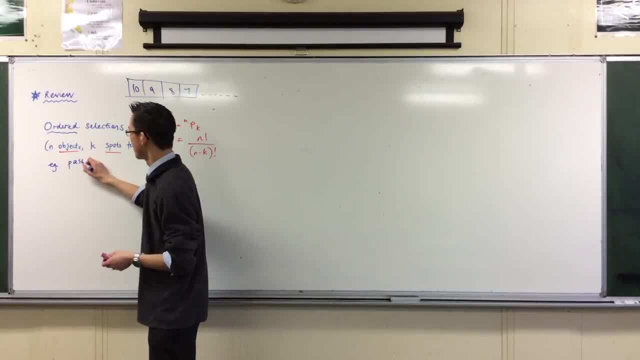 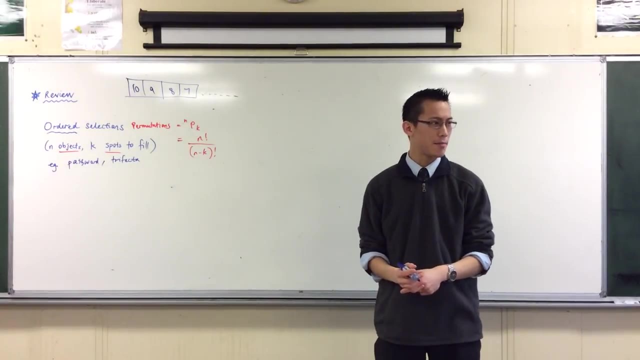 Things like a password, The order kind of matters in a password. Other things like, say, a trifecta, First, second, third, Those kinds of situations, order matters But lots of the time, and remember we're in the context of probability- 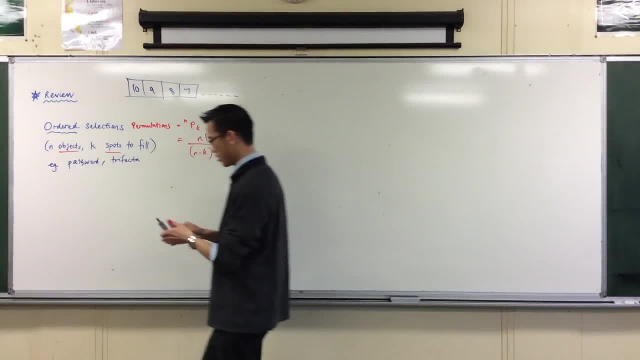 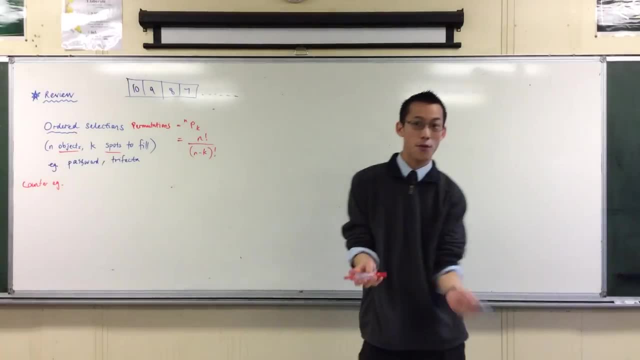 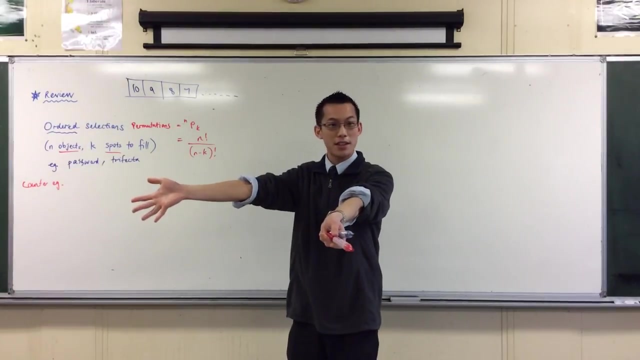 lots of the time, order does not matter, So here are my counterexamples. If you are selecting a team for a sport, I mean, just don't worry for a second about sports, where positions matter. I'm just like which four of you are going to be on this team. 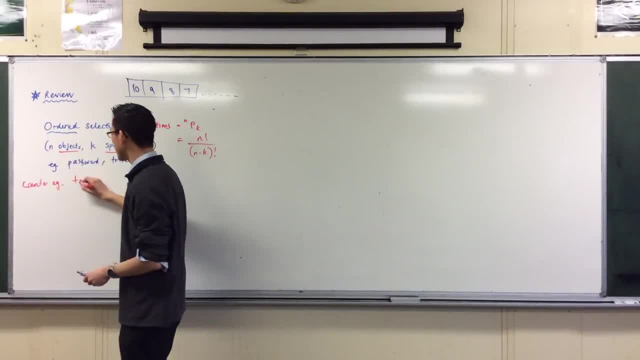 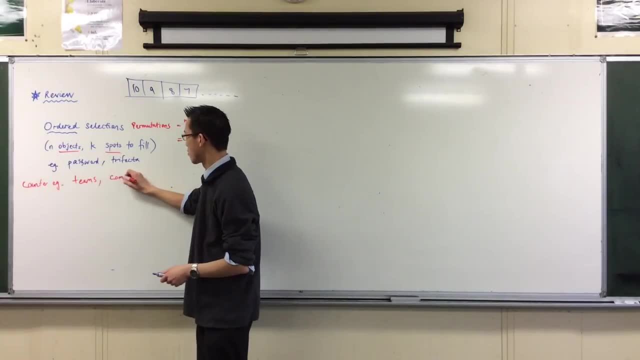 And which four of you are going to be on that team. Teams: The order doesn't really matter all that much, I just want to know who the people are. Or committees: Everyone's going to be the same on this committee. It doesn't matter which order you get picked in. 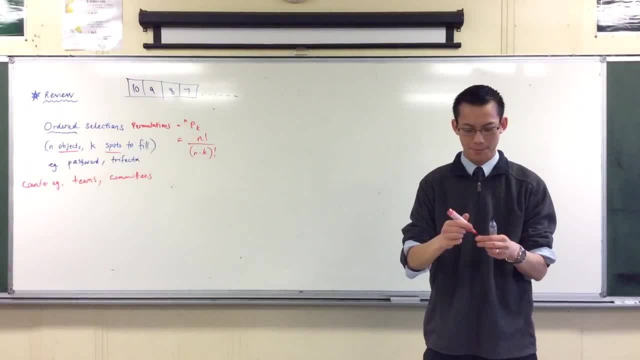 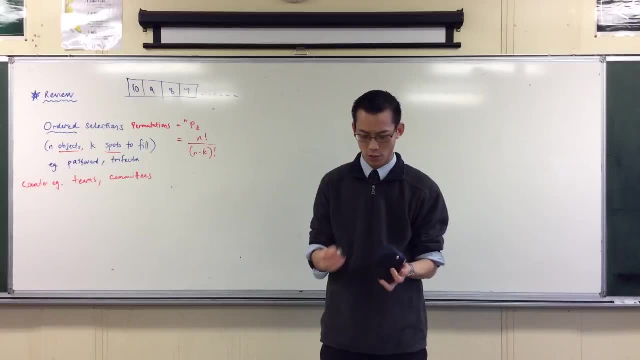 And when we're thinking about probability, for example, consider a question like a coin gets flipped. So we've looked at these and we drew probability trees or dot diagrams and so on, And one of the classic questions would be: what's the probability that you get one head and one tail if I flip twice? 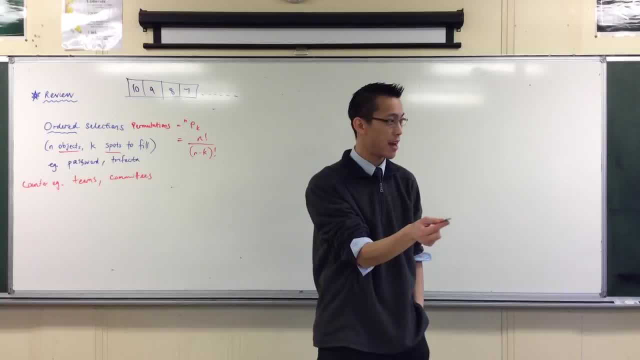 Now you don't care whether the head comes first or whether it comes second. Head-tail and tail-head are the same with regard to which ones you're interested in. So in lots of situations related to probability, we're in this kind of camp. 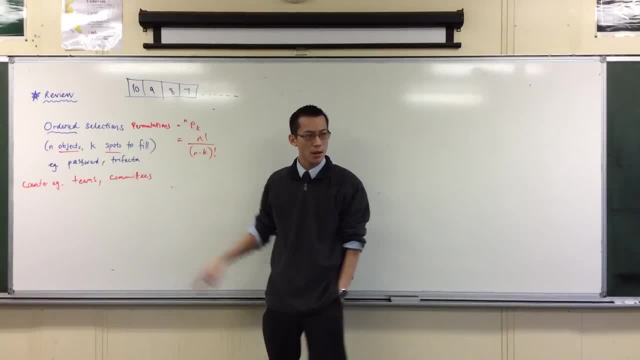 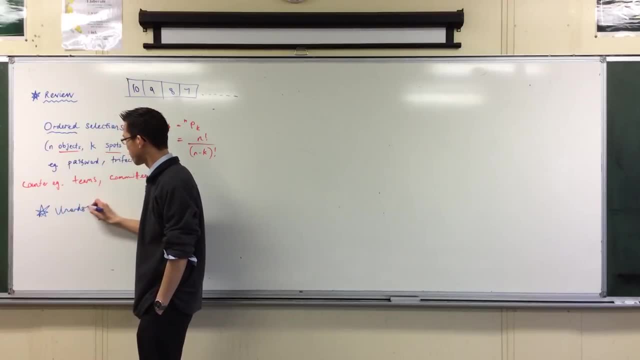 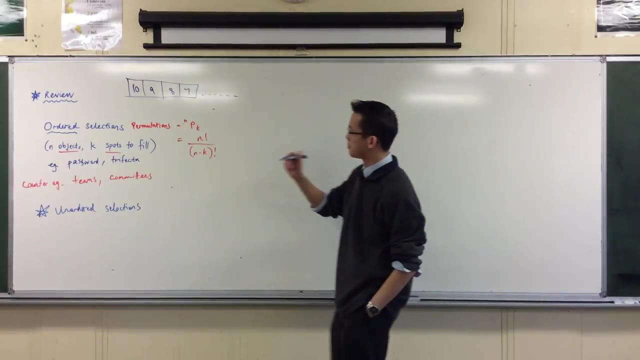 We're not in this camp, We don't worry about order. So therefore, in unordered selections, how can we relate this to what we already know? Well, let's think. Let's think of this example here. So suppose 10,, 9,, 8,, 7.. 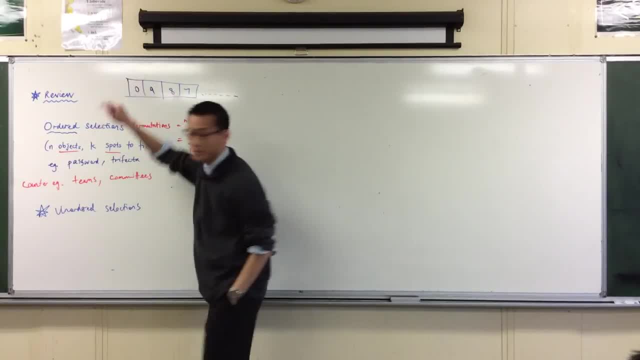 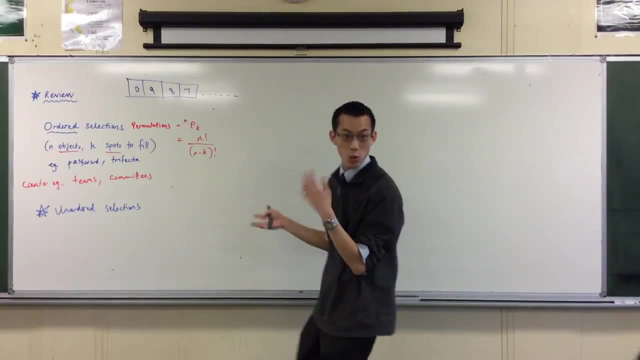 Let's make it a zero. There's a password, So I've got a password there. Now, if I don't worry about the order, that means that if I swap some of the numbers, for example, if instead of this, I have: 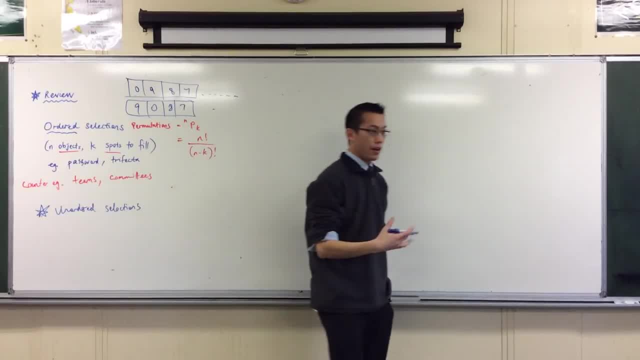 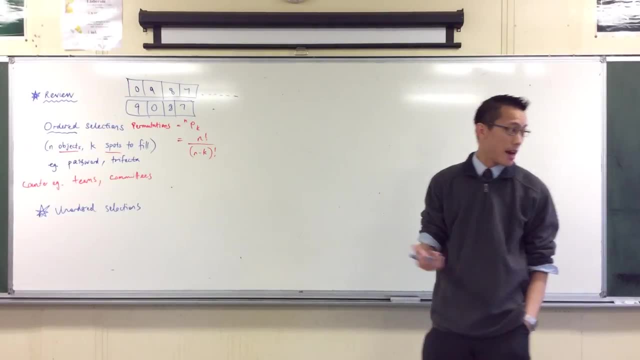 let's switch those two. if those are the same, it's the same selection, without worrying about order. You can see that there's going to be more than two ways to rearrange these same four numbers, and it'll be the same set of four numbers. 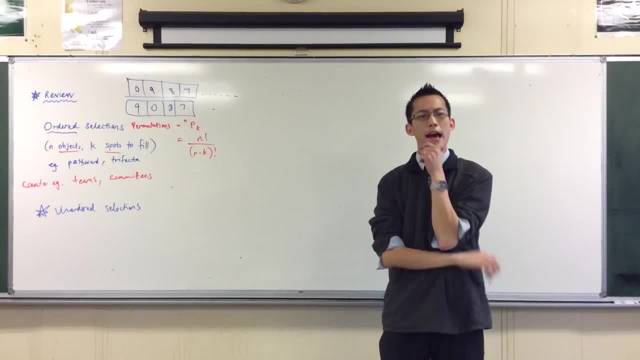 just in a different order, which I don't worry about Now. the question is: how many? How many different ways can I rearrange these four, and I'll still have the same four numbers? The answer is four. factorial, It's four, pick four. 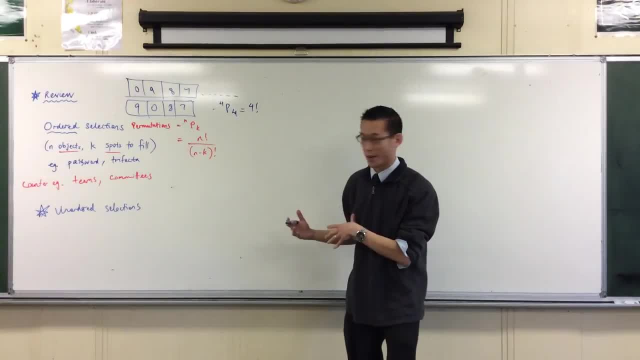 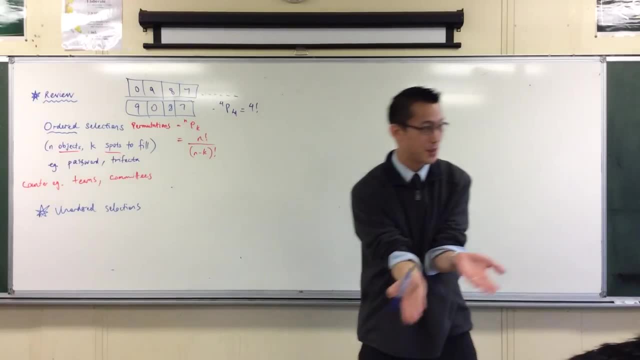 Right, So hold on a second. If I come to you with all of these different permutations we already worked out there are 10,000 of them, right? And I say, look, here are my 10,000 different passwords. 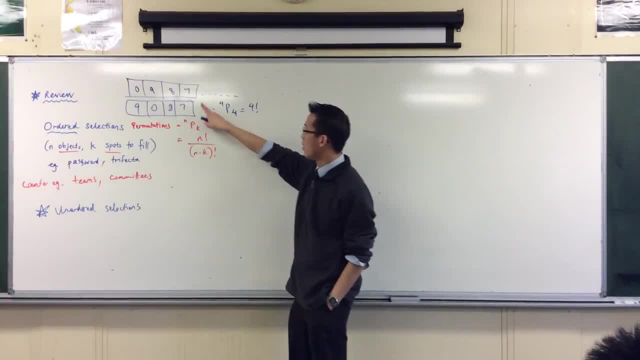 And you start to flick through, you start to look through the list and you're like: hold on this set of four numbers. you don't care about the order. This set of four numbers is the same as this one, which will be the same, as you know. 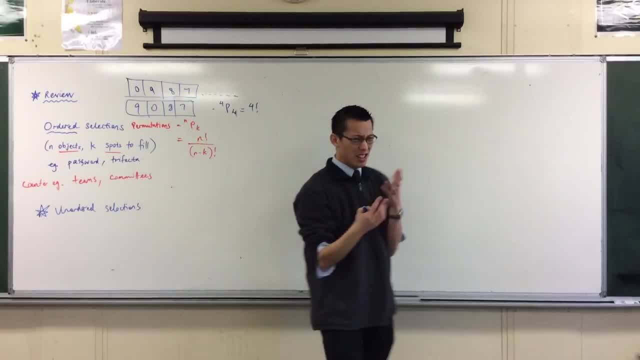 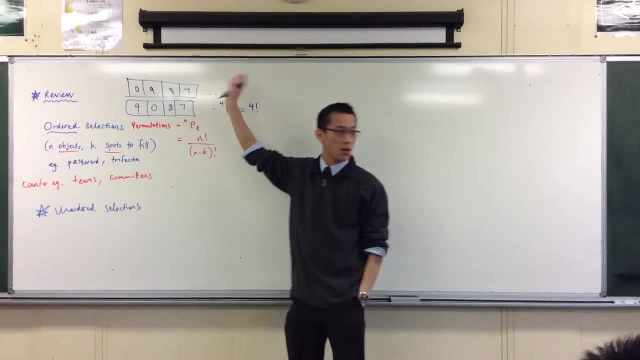 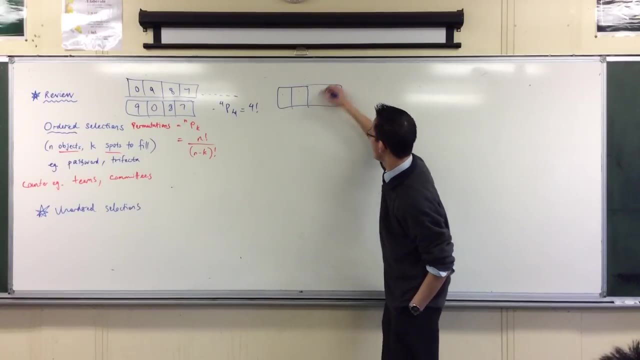 if I switch these two numbers, or switch these two numbers, and you'll be like, look, there are four times three times two, there's like 24 passwords- sets of four numbers that are all the same, right? And you repeat it every time you get a new set of four numbers, right? 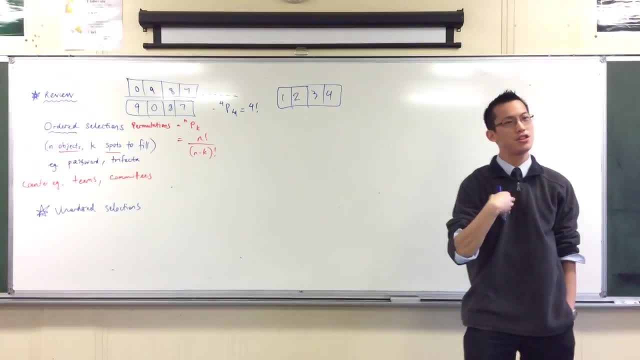 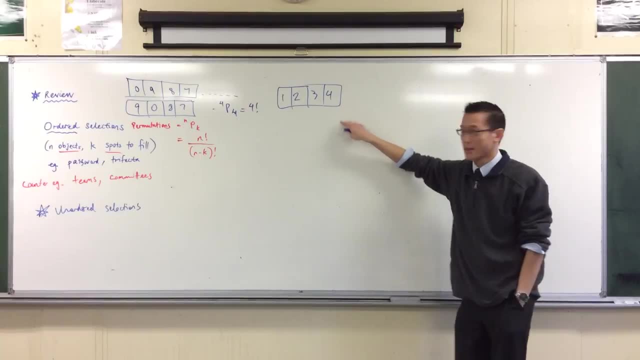 I go one, two, three, four. There will be 24 of my permutations that, for your intents and purposes, I don't care about order, they'll all be the same. There'll be another 24 of these and another 24 of the next set. 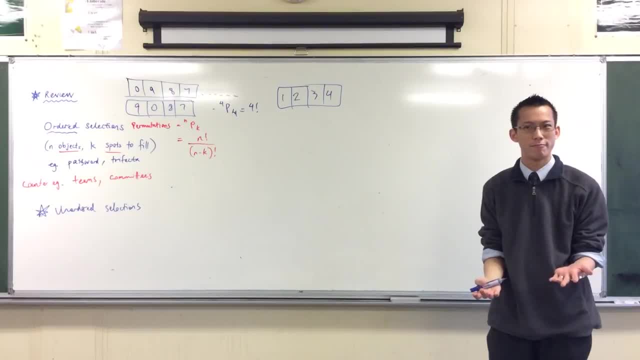 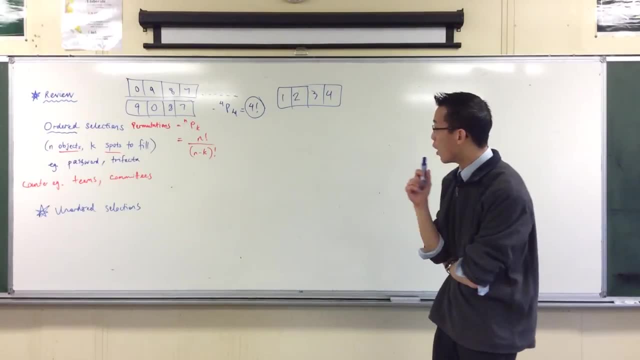 So I've overcounted. How much have I overcounted? How much have I overcounted by? I've overcounted by that 24, that four factorial okay, And obviously if I had a five-digit password, there would be even more ways. 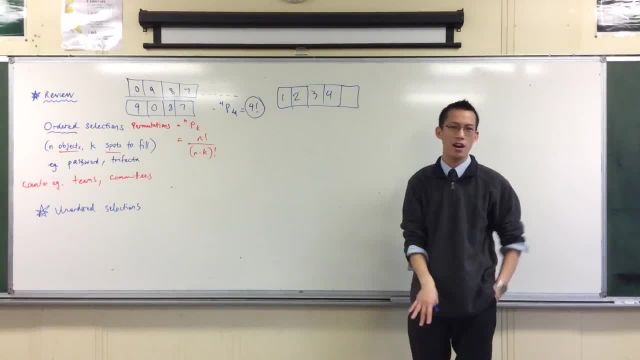 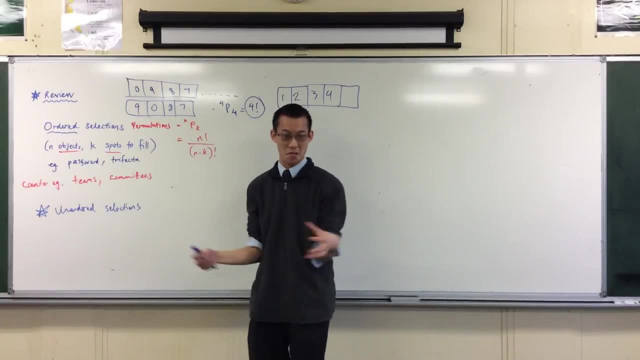 for me to rearrange these, and you don't care, because you don't care about the order. okay, So therefore, if I don't care about the order, if all I want to do is combine them in some sort of way, 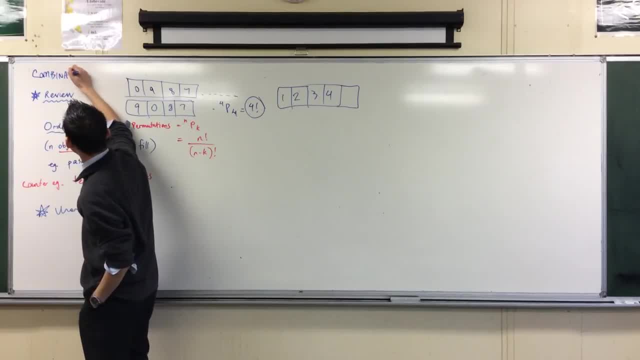 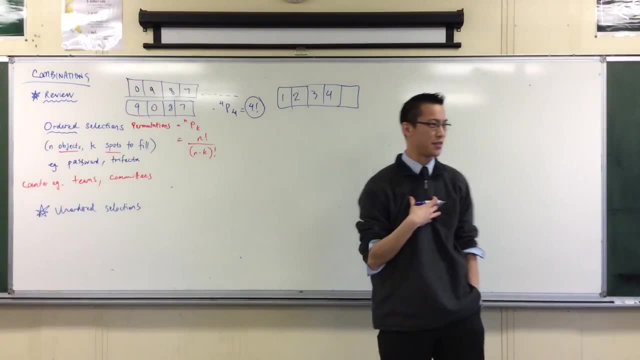 and that's what this is about. this is our counterpart to the idea of permutations, where order matters. combining. the picture I have is like in a recipe: you know, combine all of the wet elements in a bowl, You don't care where they go. 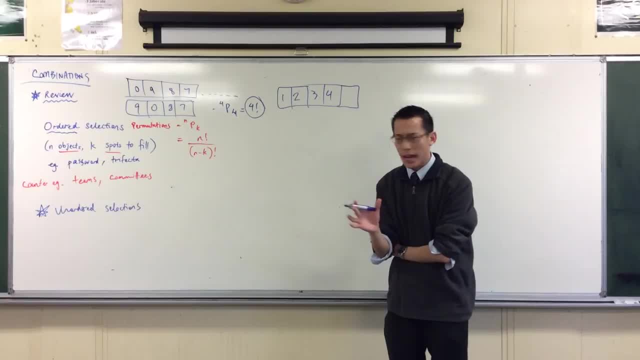 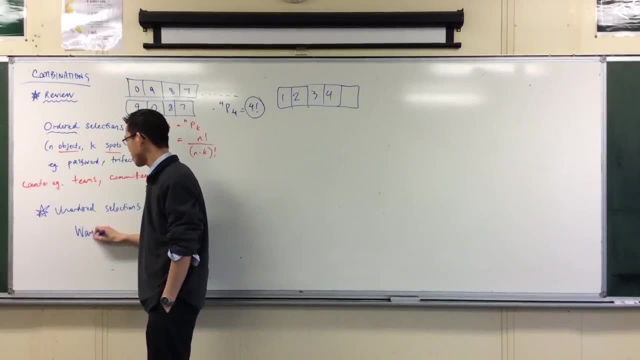 you just chuck them all in, okay, If I don't care, then I've overcounted. This thing is wrong. It gives me too many, okay, So the number of ways will start with npk. but I have to divide by something, right? 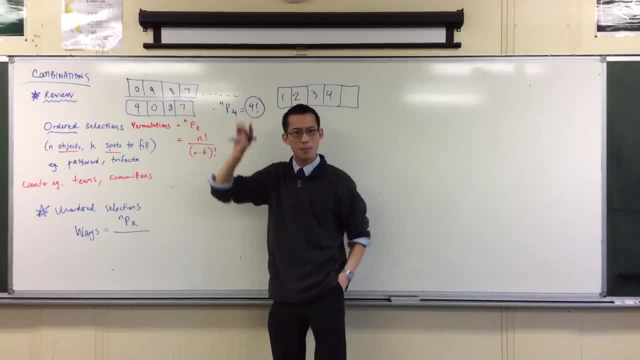 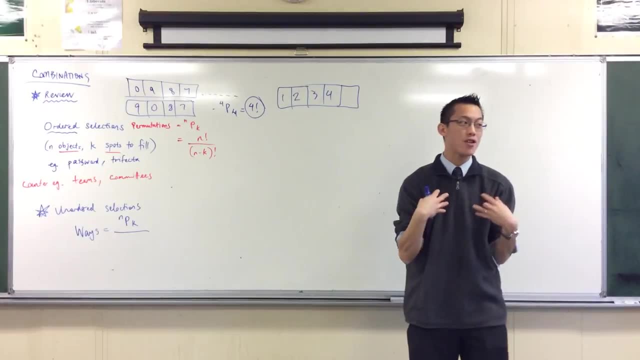 Now, in this case, I divided by four factorial. Why did I divide by four factorial? Because that was the number of ways I rearrange and you're like: I don't care, Just give it to me, just give me the numbers. 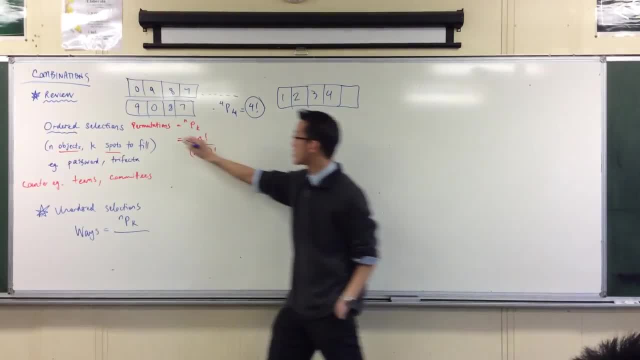 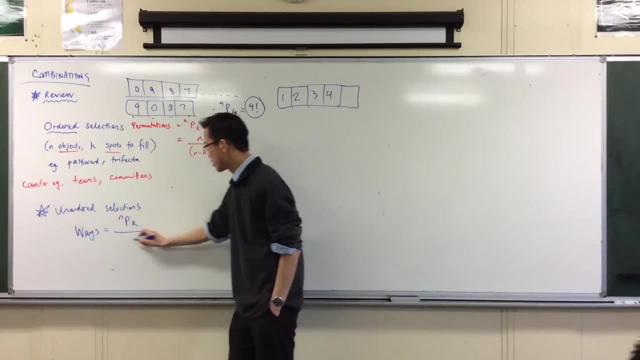 I don't worry about the order. okay, I overcounted by four. factorial. that's the number of spots I have to put them in. right, That was k. That's why it's four factorial. it's k factorial, So I've overcounted by that factor. 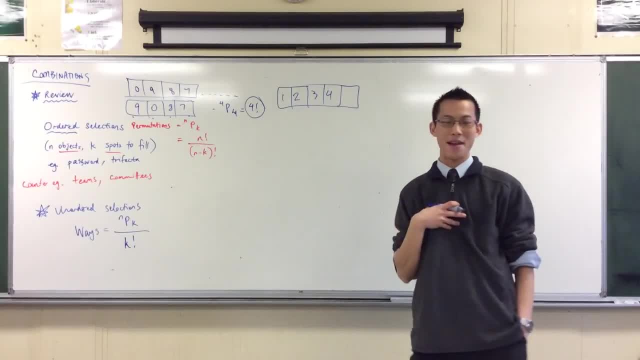 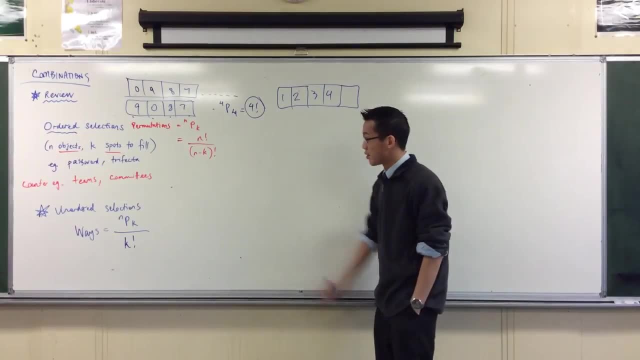 Does that make sense? So that's how we go: from my list where I care about order, because I'm OCD, to your list where you're like: I want to know which numbers they are. Order doesn't matter. So therefore, of course, 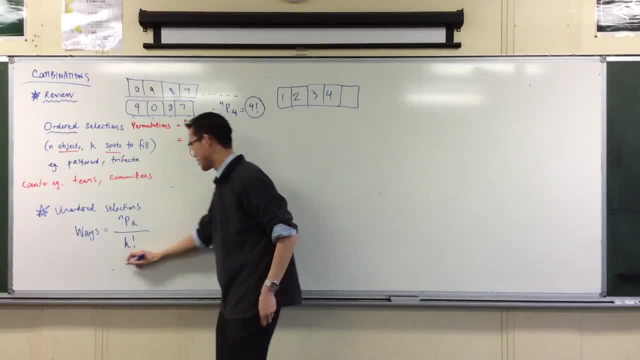 you can go back to this factorial notation and you can say: sorry, I've run out of space so I'm going to do something naughty and go across the board. You've got this guy n factorial on n minus k factorial.